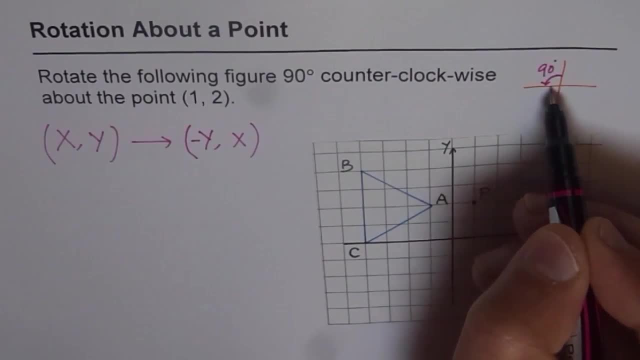 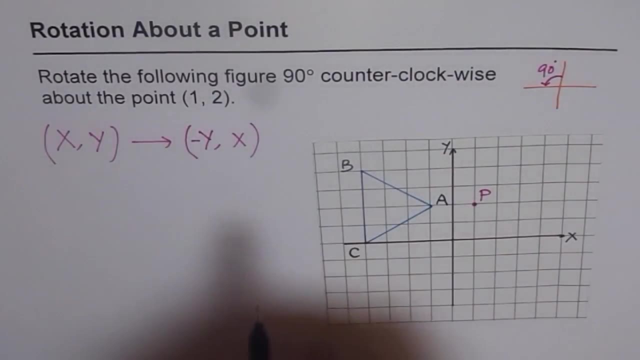 on this side and negative on the other side, and therefore we make them negative. so basically, we just swap x and y and change the y value to negative, which becomes the x value. so that is what you do. in words i can write like: what you do is swap x- y. correct, this is what you do. 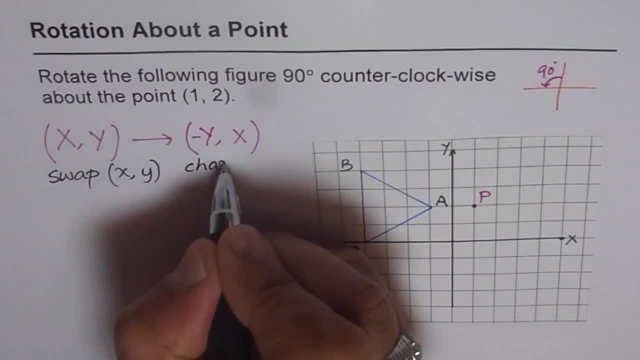 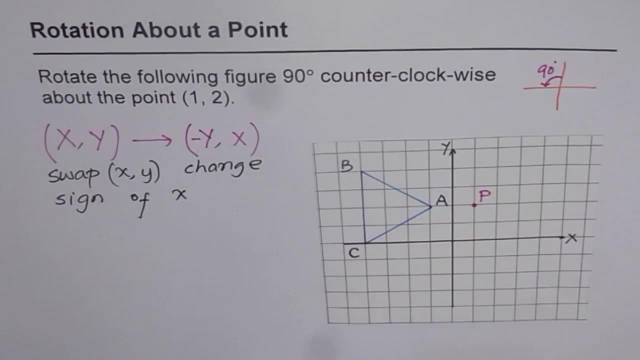 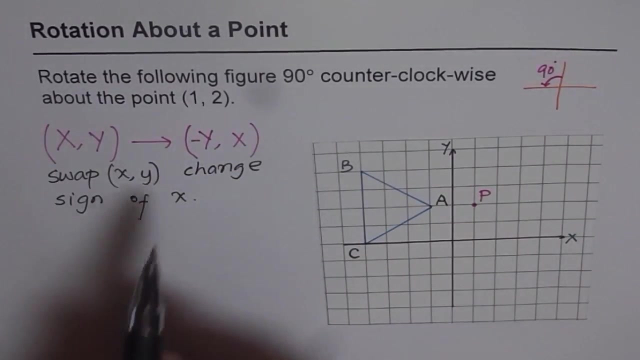 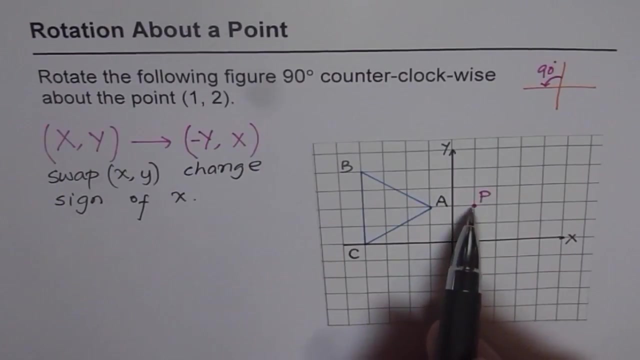 right. so you swap x, y and change sign of x. so when you swap after that, change the sign of x. so that is another way of saying the same thing. so this is what you do when you do rotation about the origin. right now, here we are rotating about a point which is not the origin, so we cannot apply this rule. 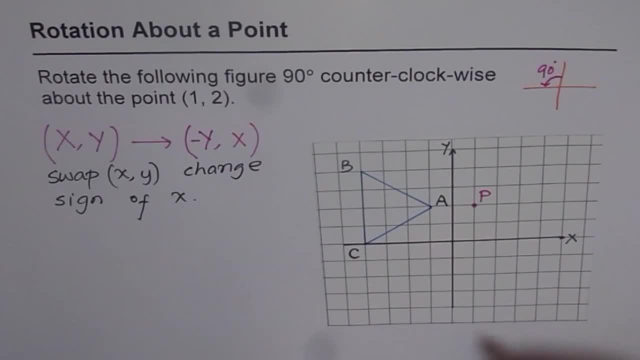 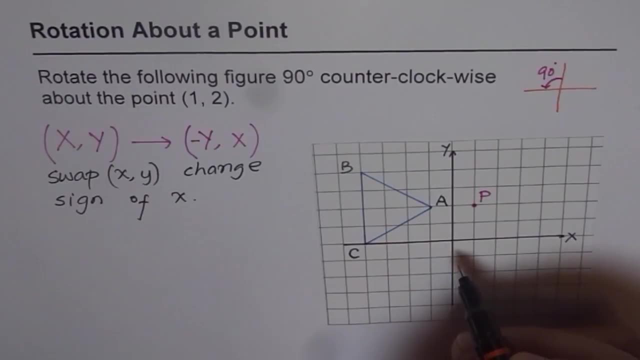 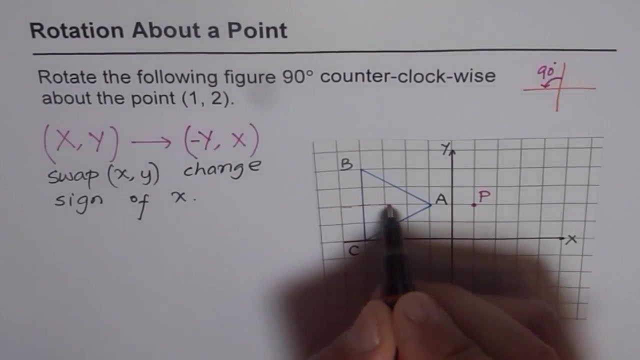 that is tricky, right? so let us see how to apply the rule and do our work. so what we will do is we will make p as our origin, right, so we'll modify the plane itself. so think about a coordinate axis like this here. let me draw this as the x axis. do you see that? so what i'm doing is i'm shifting my 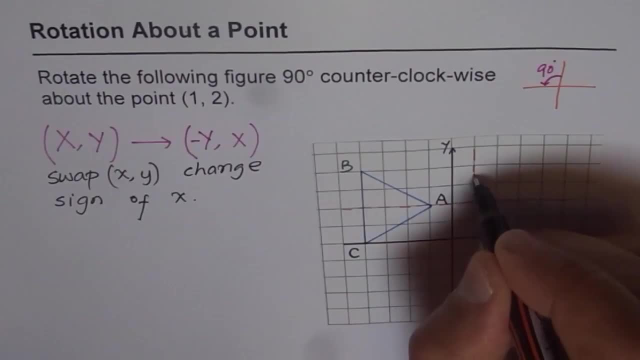 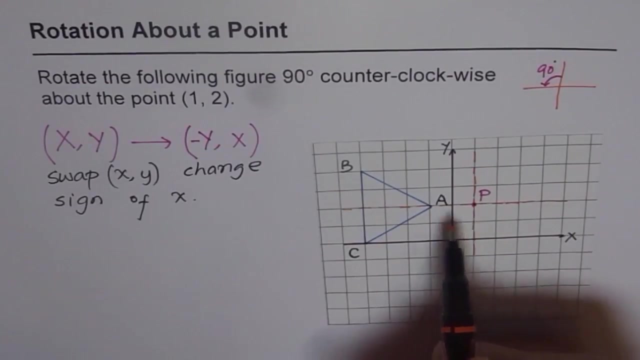 origin and i'm shifting it to the point around which we have to rotate counterclockwise. you see that. so this is a shift. now i've made a new coordinate plane with p at the origin, correct. now let us see the whole triangle from this new perspective. 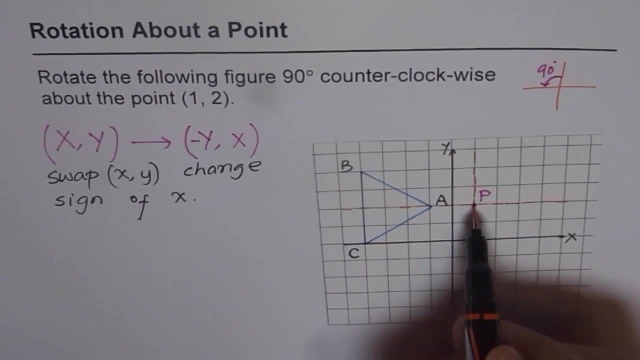 as p being the origin. now, if p is the origin, then i can apply this rule. so that is the beauty. so let's see how to apply the rule now. if, if p is my origin, then what are the coordinates? of point a will be 1: 2, since we are going left minus 2 right as far as y value concerned. we are not moving up. 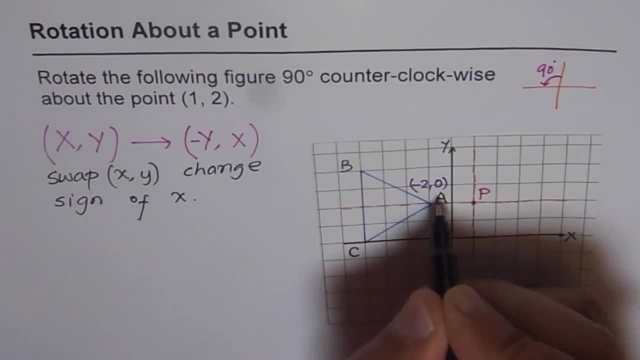 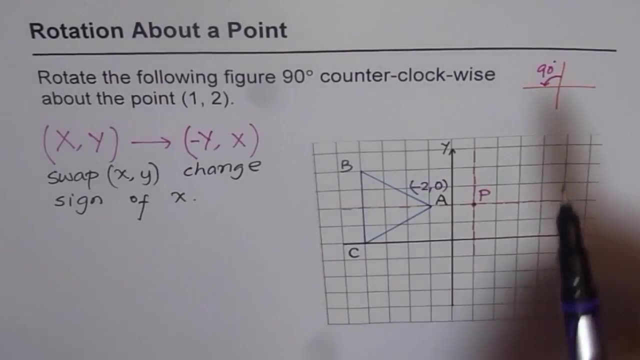 or down. so it is just 0, right. so the coordinate of point a from p is minus 2, 0 to rotate is counterclockwise 90 degrees. we have to swap right. so once we swap, what do we get? we get a dash. so 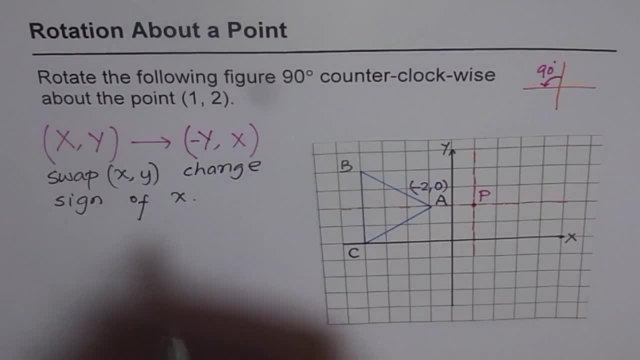 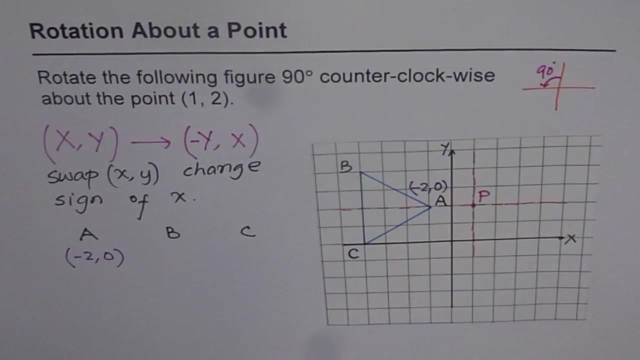 let me write down our modified points first here, right? so i'm writing a, b and c and i'm writing here my modified coordinate points. and modified coordinate points are minus 2 and 0 for a. now, if i have to do 90 degrees counterclockwise, 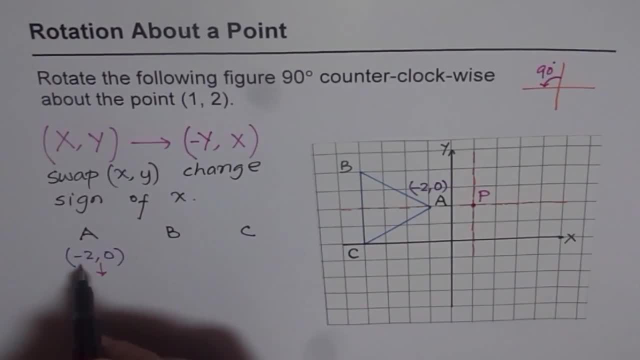 what should i do? i need to swap it and make or change the sign of x. so once i swap, that means i'm bringing 0 here minus 2 there, correct. so what do i get? i get 0 with the negative sign. it's not a good practice to write. 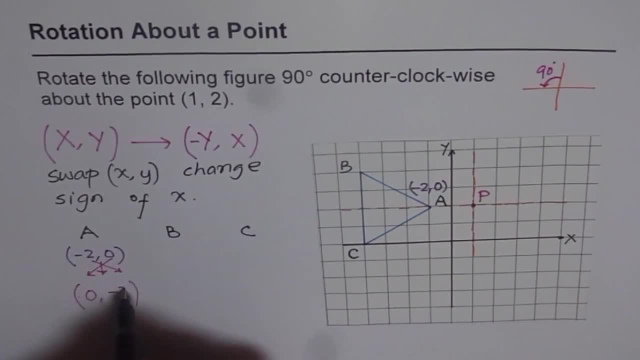 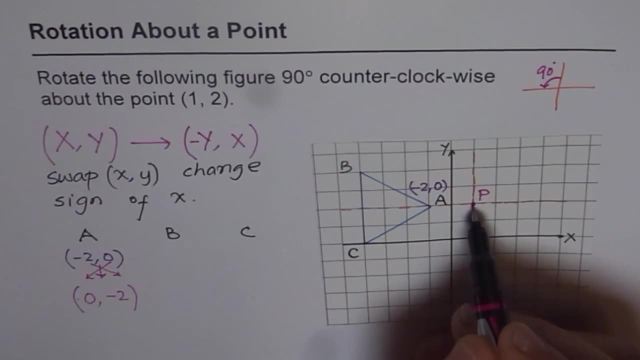 negative. so i'm leaving that and this minus 2 comes here. so that is my new coordinate: from p as center. do you see that? so from p as center let's go to a point 0 minus 2. so 0 means in x direction we are not moving, but in y, 1, 2, so we get a point here. do you see that? and this point becomes a dash. 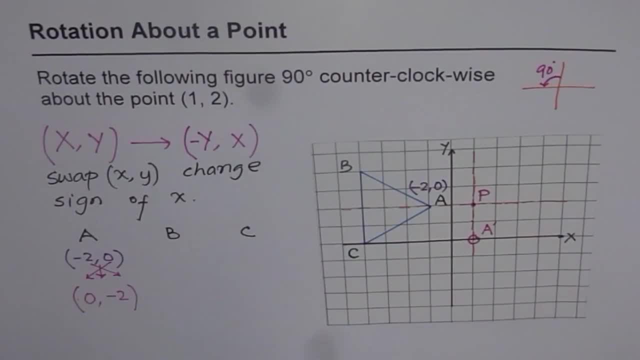 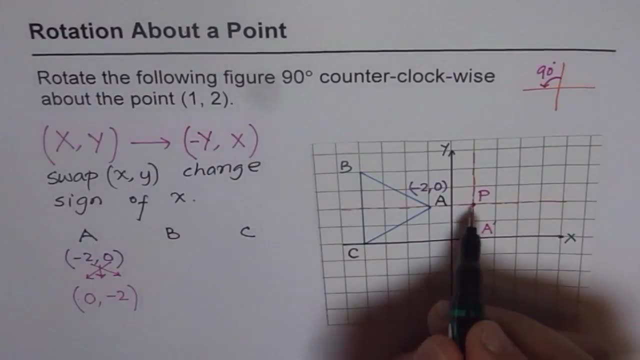 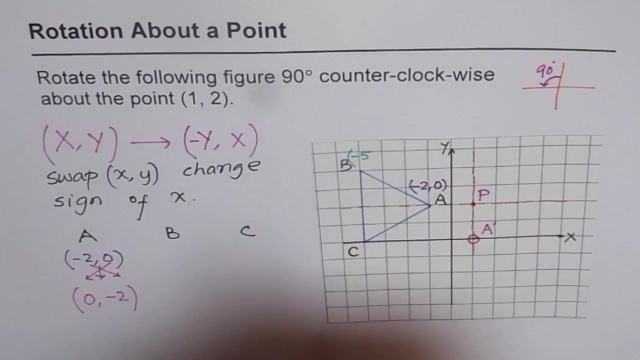 for us. let me write down the coordinate of point a and this point becomes a dash for us. let me write a dash now. similarly, let's do now point b. see how we are doing it. let's do it again to reach b from p one, two, three, four, five units left means minus five. do you see that dash? and one, two units up. 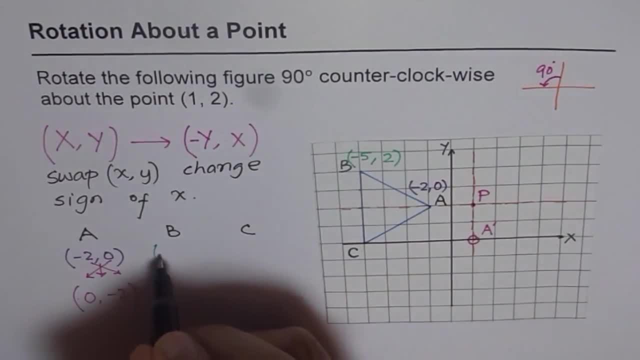 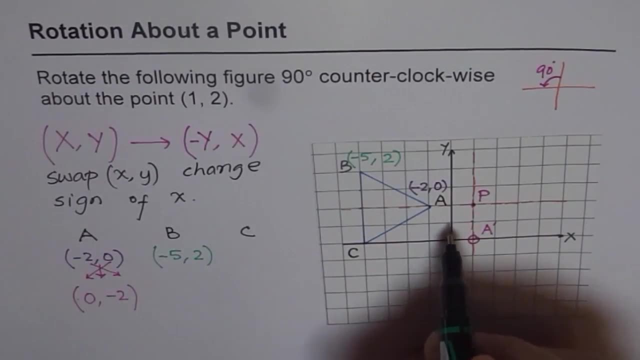 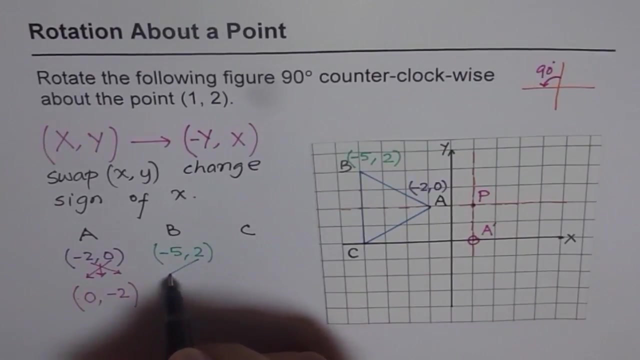 that means plus two, so coordinates of b will be minus five and two. this is with p as the origin. and now to rotate it 90 degrees counterclockwise. what should we do? let us swap it right. so we'll swap this and this and change the sign for x. that is the rule, correct? so once we do that, what do we get? 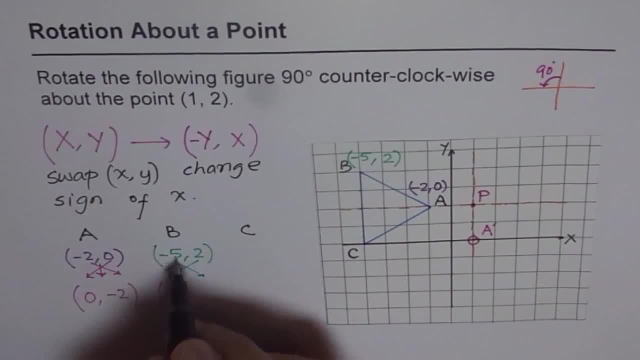 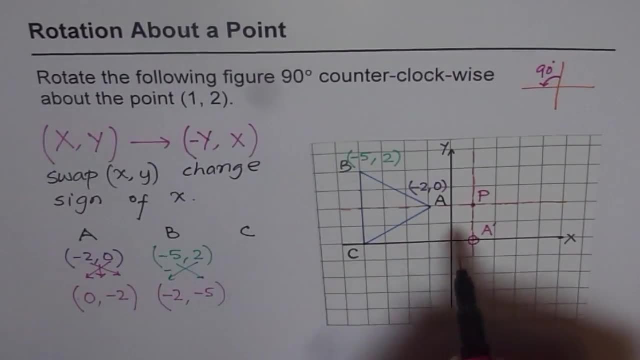 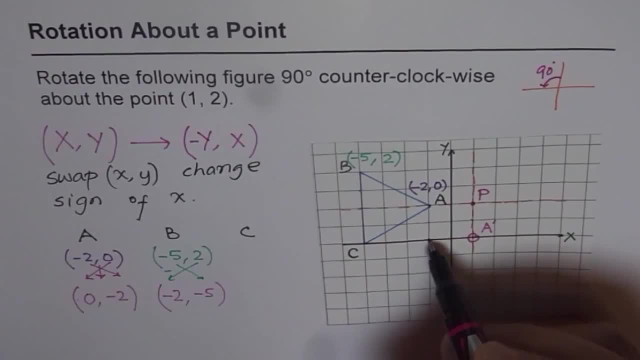 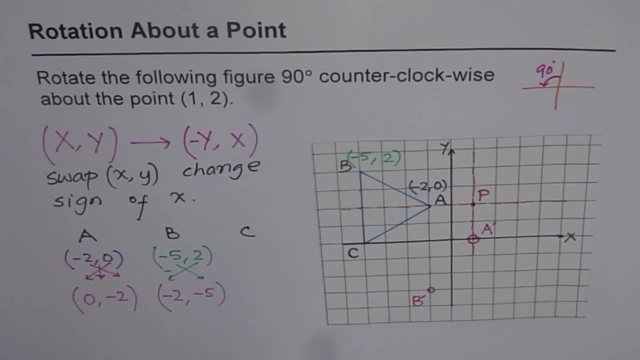 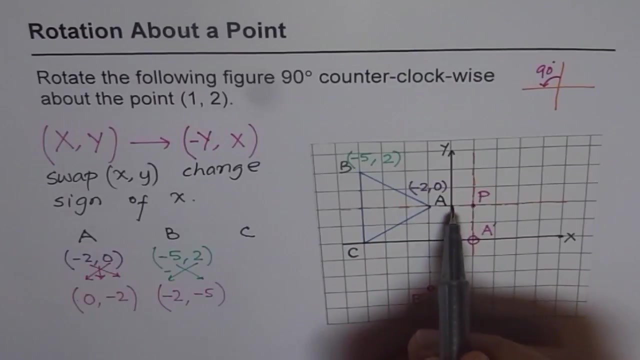 two means one, two minus five means one, two, three, four, five. so there you are. so that becomes your by yo. point b. let me call it b dash, correct. so we get two points. now let's try for c. now for c. let us say that the point c is from p as the origin: 1, 2, 3, 4, 5 units to the left, so it is minus 5, let me. 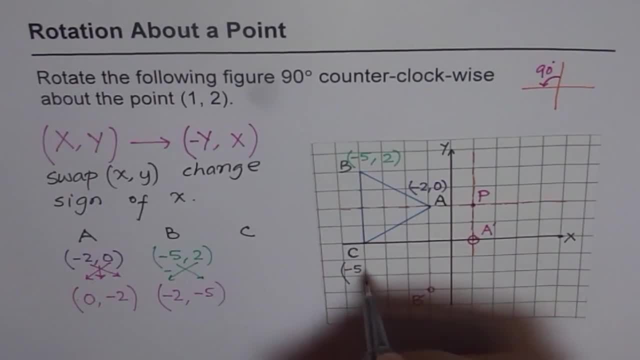 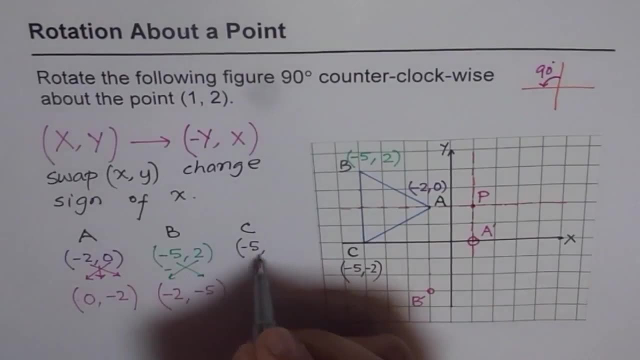 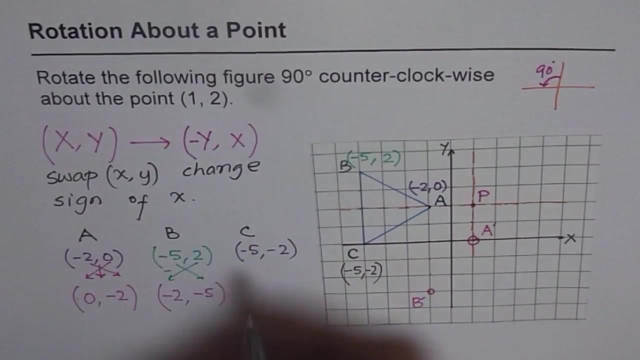 me write minus 5 here and 1, 2 units down, minus 2, 2 units down. so the coordinates of point C are minus 5 minus 2. now we want to rotate it 90 degrees counterclockwise. what should I do? swap and change the sign, swap without changing the sign and we get our new coordinates, which are: 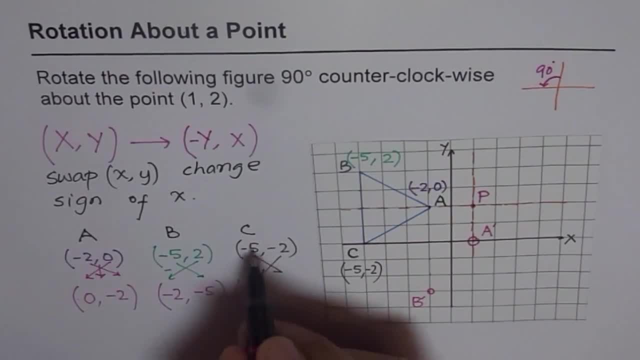 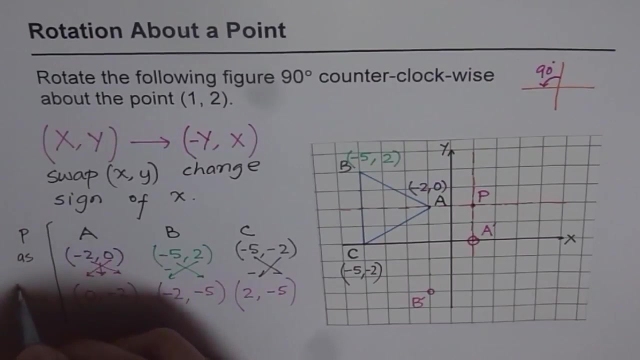 if I change the sign I get plus 2, here plus 2 and here we'll give minus 5 as such. so these are my new coordinates: 2 minus 5. and remember these coordinates are all from P as origin, right, P as origin, so new plane. do you see that new coordinate plane? so we'll go. 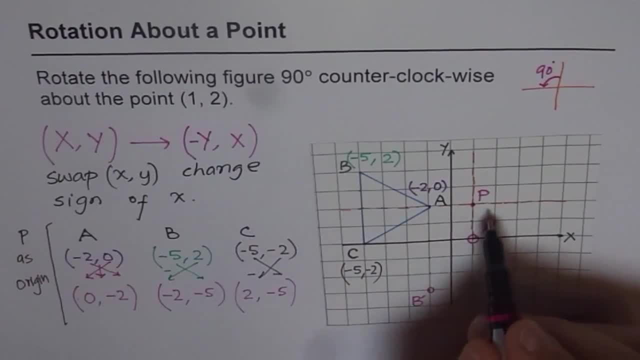 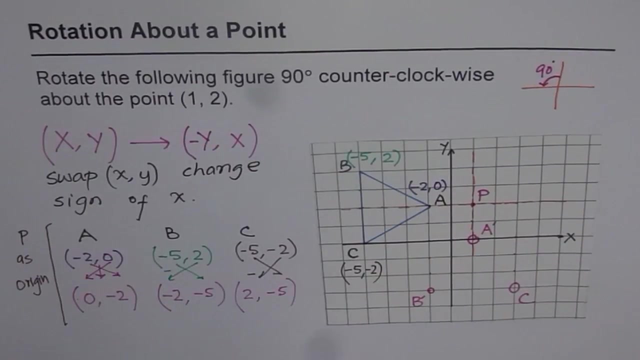 from P, 2 comma minus 5. 2 means positive 2, 1, 2 units minus 5 down 5, 1, 2, 3, 4 and 5. so we get our point C here. do you see that? so these are our new points and now we can join them to get the answer right. so once we join, 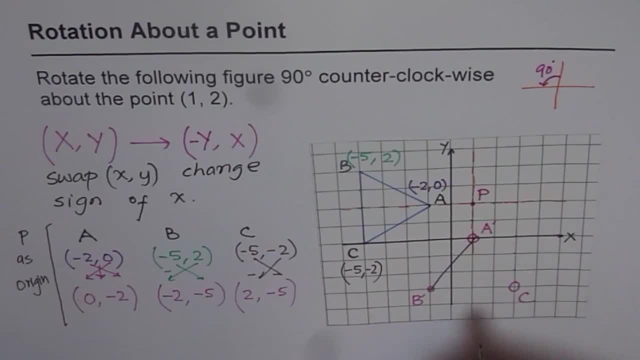 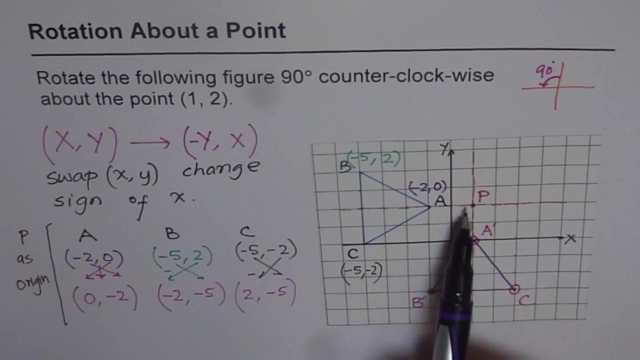 what do we get? we get a triangle here. this is A to B, B to C and then from A to C. so this is how we can rotate a given figure around any point apart from origin, Any point it works. Go through it once again. So the idea is: whenever you are rotating 90 degrees counterclockwise-